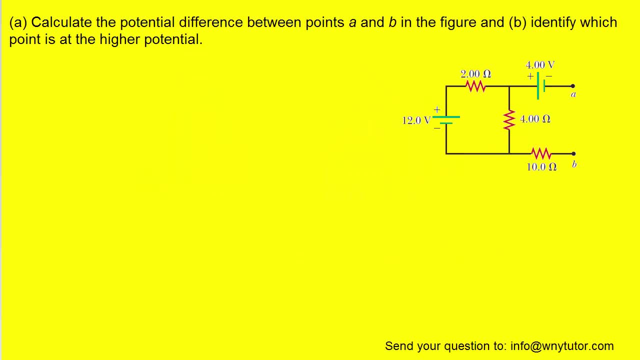 If you haven't done so yet, please pause the video and try to solve the question on your own before listening on. What's important to understand in this question is that there is a gap between point A and point B and because of that gap, current will not flow through this portion of the circuit that we're 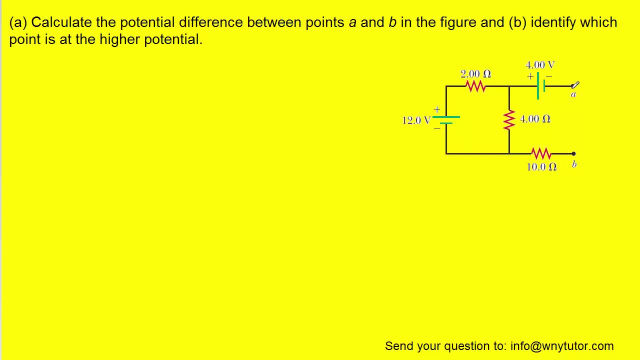 outlining with the pencil. Now, of course, if we were to connect point A to point B with a wire, then we would have a nice closed circuit and current would indeed flow around that portion of the circuit. But again, in this case that simply will not happen. So, in essence, we can actually cut out this portion of the circuit. So 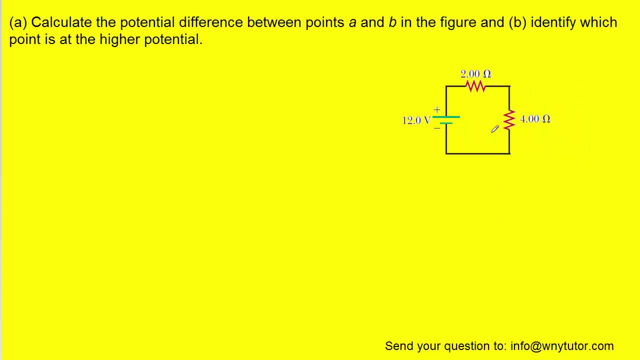 let's go ahead and do that so that we can simplify the problem. So what we're left with is a simplified circuit that has two resistors that are in series with one another, And we know that when resistors are in series with each other. 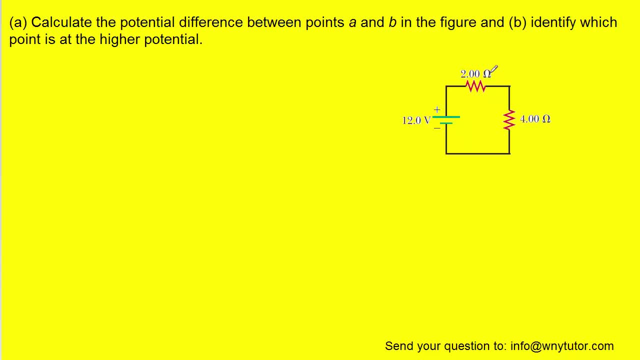 we can combine them with one another and we can do that. So let's go ahead and them by simply adding their resistances. So we're gonna go ahead and combine the 2-ohm resistor with the 4-ohm resistor by adding them together and creating a 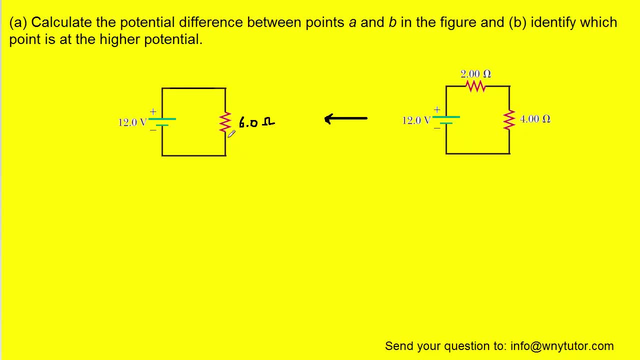 so-called equivalent resistor. And so, now that we've simplified the circuit, we can turn to Ohm's law to calculate how much current is, overall, flowing through this circuit. And Ohm's law tells us that the current is equal to the potential difference supplied by the battery divided by the equivalent resistance of 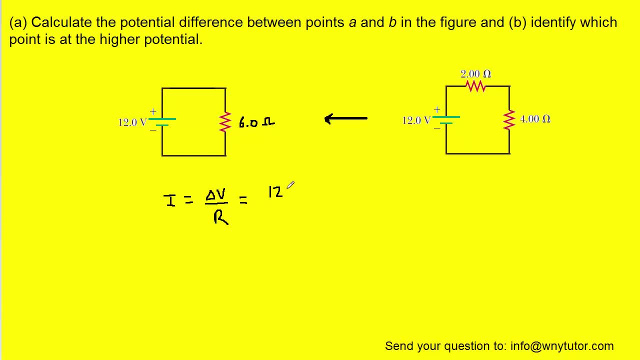 our circuit. So we can see from the diagram that we have a 12-volt battery and then we have the 6-ohm resistance. So when we divide these quantities we get a current of 2 amps, And so that's how much current is going to be flowing around. 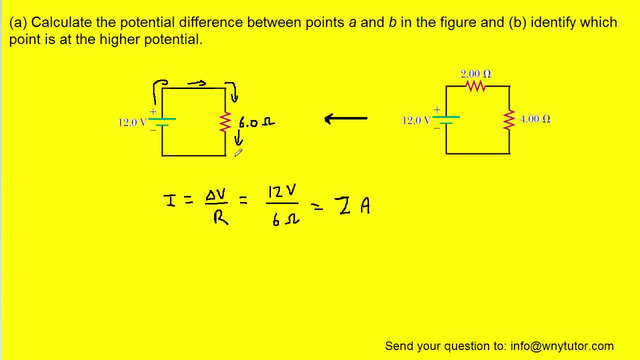 the circuit in both the simplified version of the circuit and also the more complex version of the circuit over here. So we're gonna go ahead and draw the current in Now. in order to calculate the potential difference between points A and B, we actually have to go back to the original version of the circuit, because 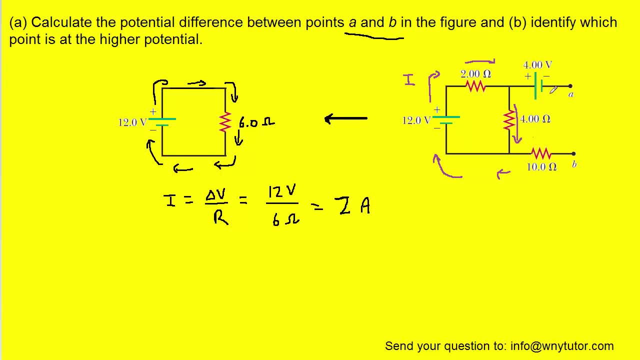 that's where we could actually directly connect to this again, But that way this where we could actually see points A and B. So we've put back the portion of the circuit that we removed originally and what we're gonna do is start at point A. 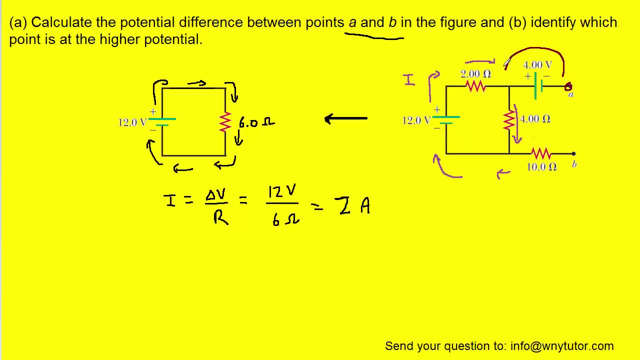 and we're gonna work our way over to point B by following this path outlined in the brown color, And as we go around this path from A to B, we're gonna be keeping track of the potential changes. So again, starting at point A, we encounter the battery. 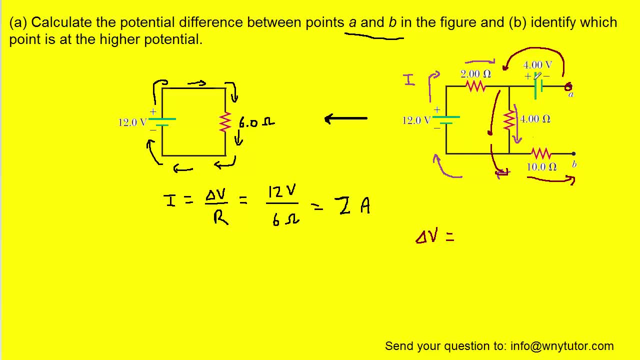 and notice that we would be moving from the negative terminal to the positive terminal of the battery. That's going to represent a positive potential change of four volts. And then, as we continue our journey through the brown colored path, we encounter this resistor and notice that we're flowing with the current. 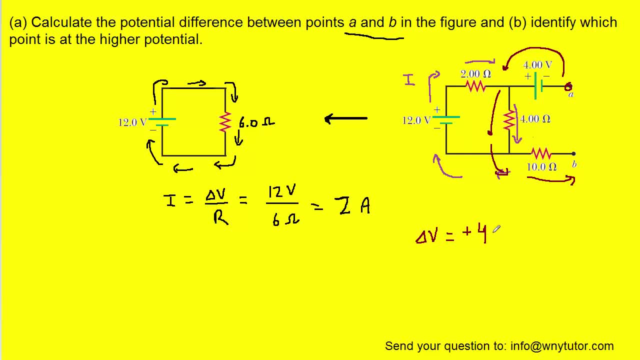 as we move along this path. When you're flowing with current, the potential difference across that resistor will be negative and it will equal the resistance of four ohms times the current that was flowing through there, and that's the current that we had determined earlier. 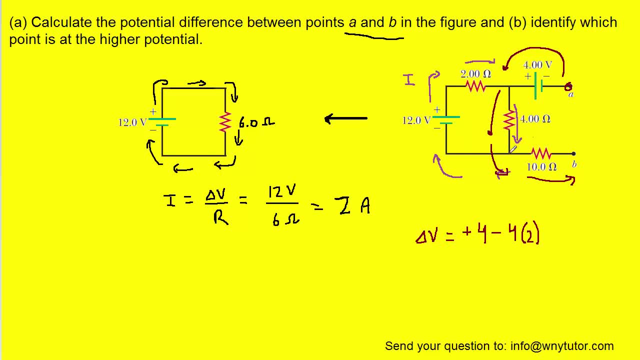 to be two amps, so we'll plug in two there. We then continue our journey to point B and we encounter this resistor. but remember: there is no current flowing through this resistor and so there will be no potential change across that resistor. 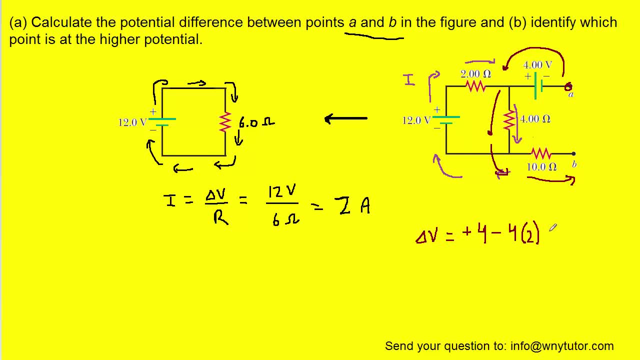 So we can basically just skip right over it to get to point B, And when we arrive at point B, we can actually simplify this and we end up with four minus eight, which will be negative four volts. That's going to be the potential change. 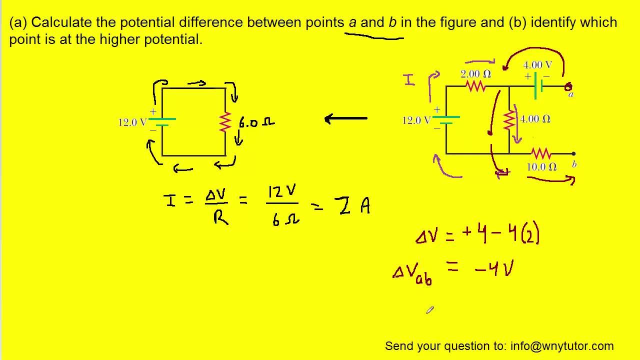 as we move from point A to point B And the question probably wants the magnitude of that potential difference. so you could just take the absolute value of both sides and that shows us that the potential difference magnitude from point A to point B is four volts. 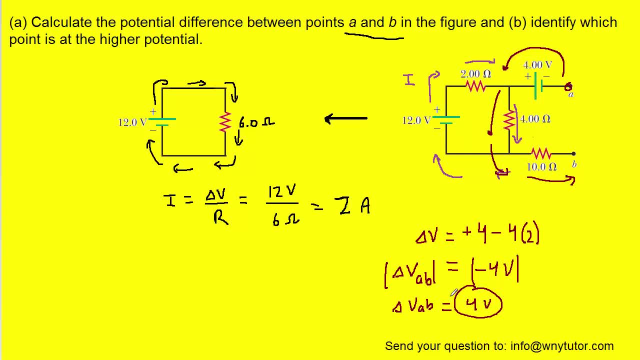 so this would be the correct answer to part A Now, since technically the change was negative. what that indicates is that the potential at point A was actually higher than the potential at point B. because of that negative sign, It's almost as if we were rolling down a hill. 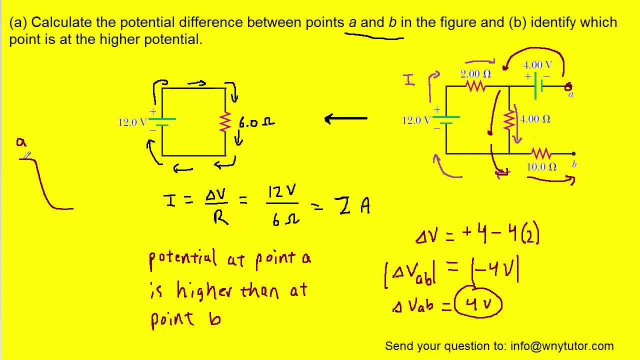 And point A, where we started, was higher up in potential, Point B would be lower, And so we can see, as we move from point A to point B, we have a negative potential change because of the fact that point A has the higher potential. 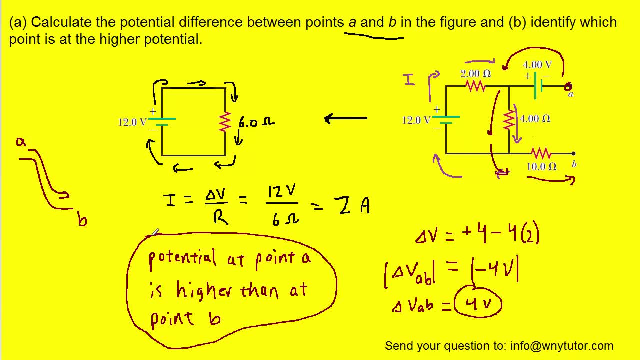 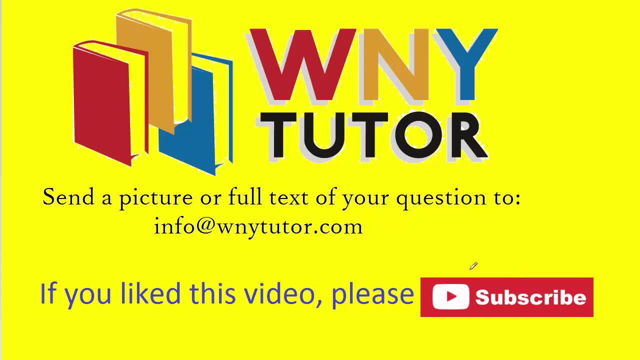 So this would actually be the correct answer to part B of the question. Thanks for taking the time to watch the video. If you liked it, please click the thumbs up icon and also subscribe to the channel so you can stay tuned for other videos.